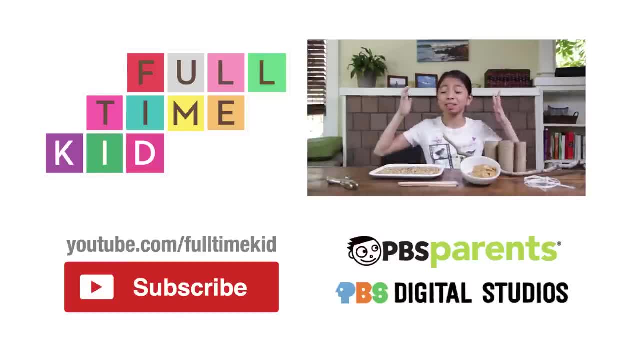 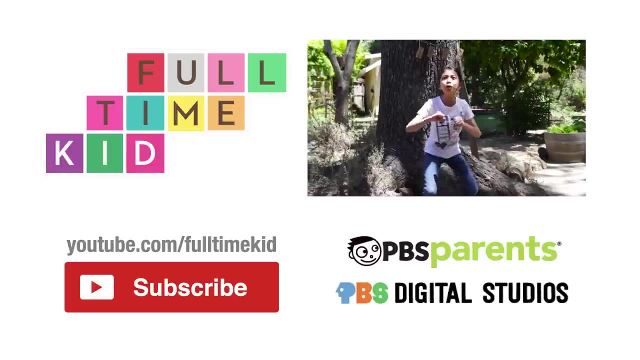 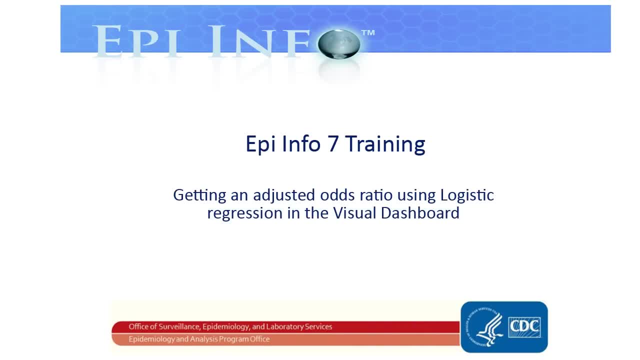 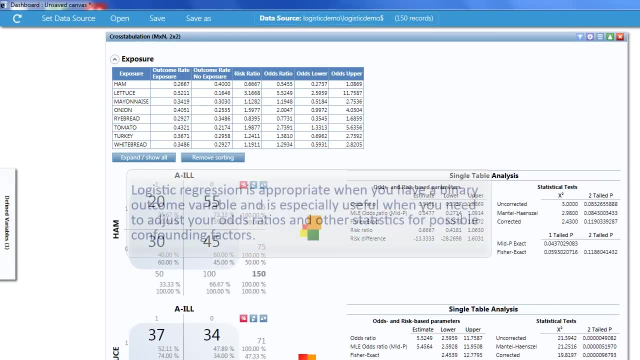 Welcome to Epi Info 7 training. In this video you'll get an adjusted odds ratio by using logistic regression in the visual dashboard. Logistic regression is appropriate when you have a binary outcome variable and is especially useful when you need to adjust your odds ratios. 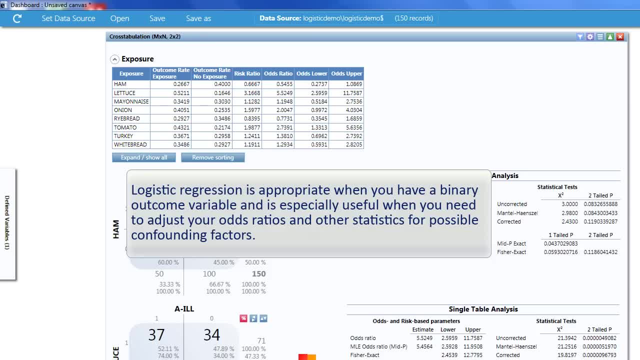 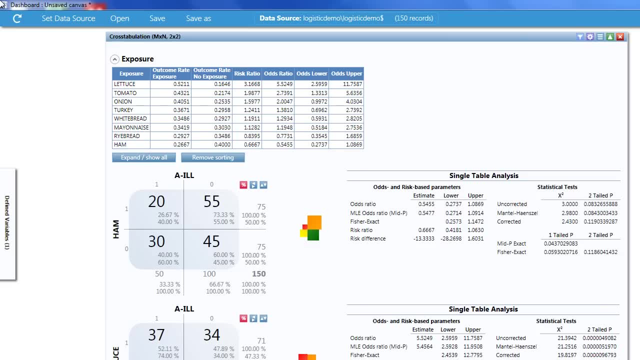 and other statistics for possible confounding factors. We have the visual dashboard displaying the results of a group of two by two analysis results. These results show three foods that could be our vehicle for food-borne illness – lettuce, tomato and onion. So we'll look at all these together in a logistic regression. 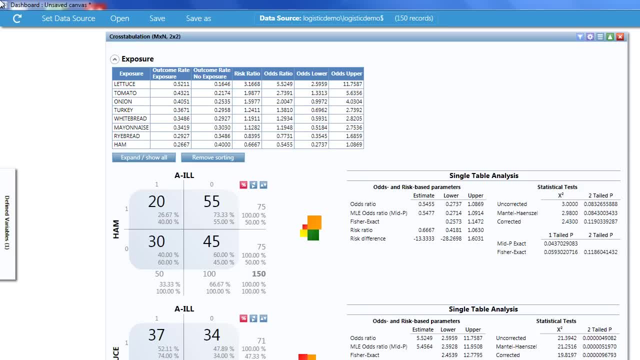 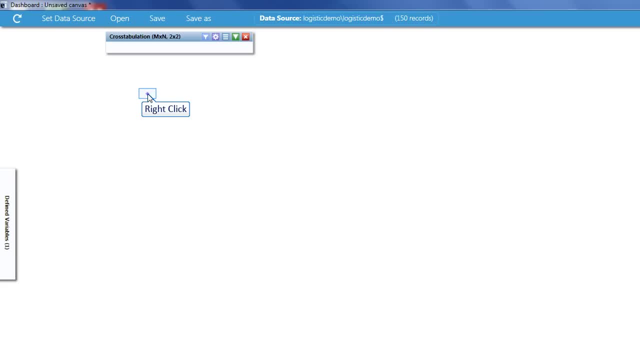 model to see if any of them are significantly associated with illness. First we'll minimize the two by two gadget. Then we'll right click on the dashboard again We'll navigate to Add Analysis Gadget, Advanced Statistics and then Logistic Regression. 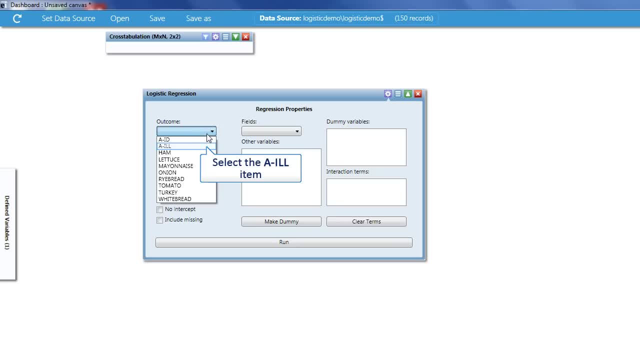 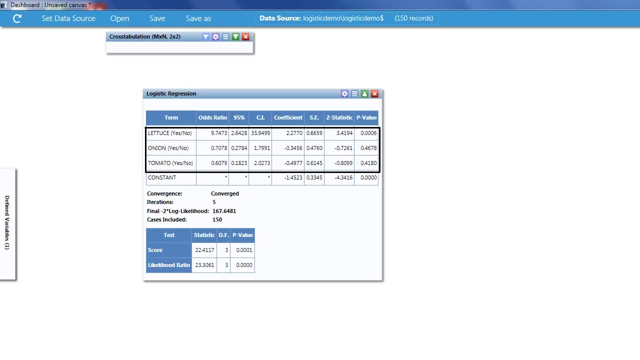 My outcome is ill and I will choose those three suspect foods: lettuce, onion and tomato. I'll click Run and minimize the dialog box. There's a row for each of the suspect foods and the first three columns include each food's. 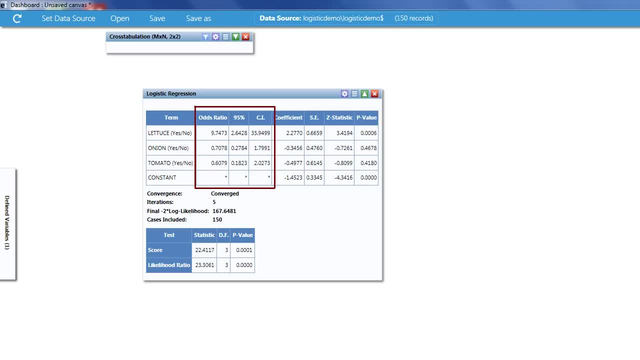 odds ratios and confidence intervals. Now, lettuce still has an odds ratio greater than 1 and a confidence interval that is significantly greater than 1.. Tomato and onion don't have odds ratios significantly different than 1.. We now think lettuce has an odds ratio greater than 1..